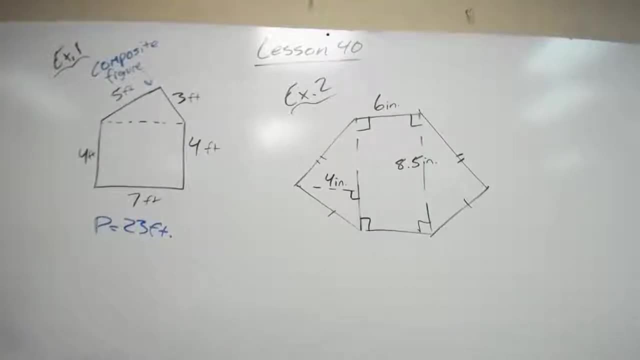 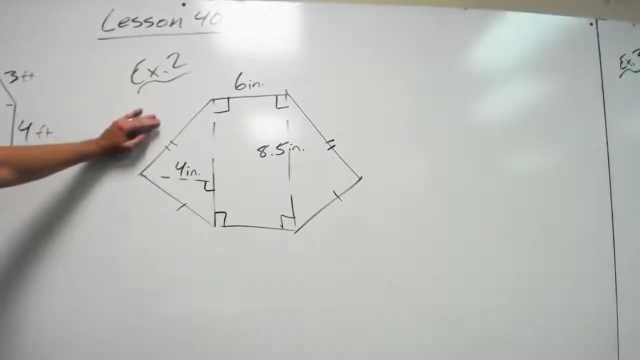 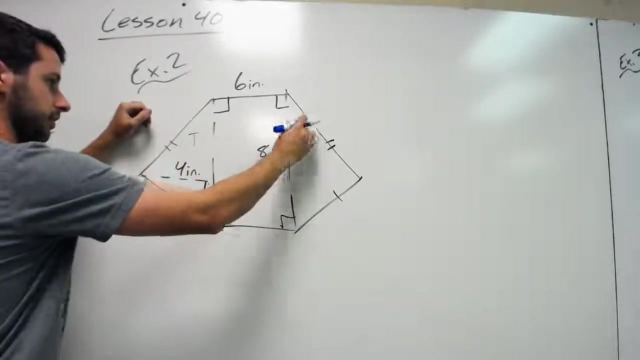 That's very basic. They're not going to be that easy all the time. But let's look at area of composite figures. Area can be a little trickier. So if we're finding the area of this composite figure, what I need to do is find the area of this triangle. this triangle. 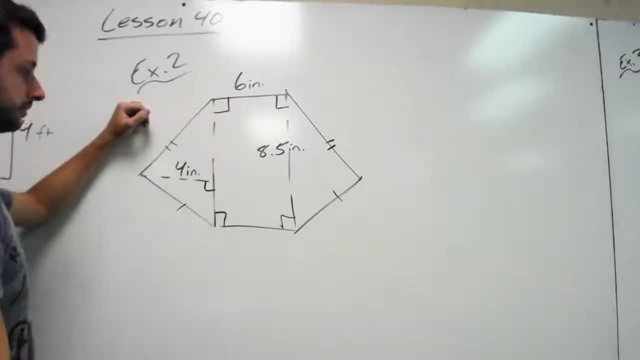 and this rectangle And then add them all together. So the first thing I'm going to do is find the area of this triangle. I'm going to find the area of this triangle. Well, 4 inches right here- Notice, this is perpendicular. 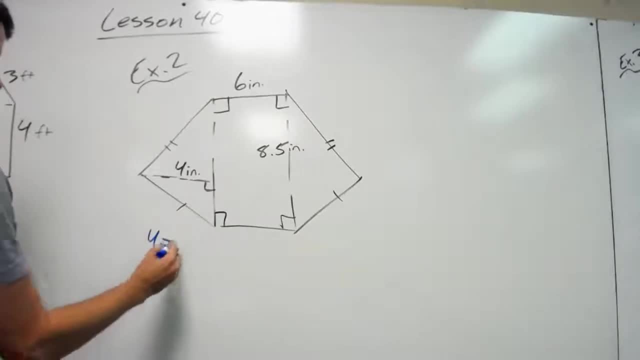 Since it's perpendicular, 4 is going to be our height. Now, the 8.5 is written over here, but we know that these are congruent And so therefore, this side is also 8.5.. And so 8.5 would be our base. 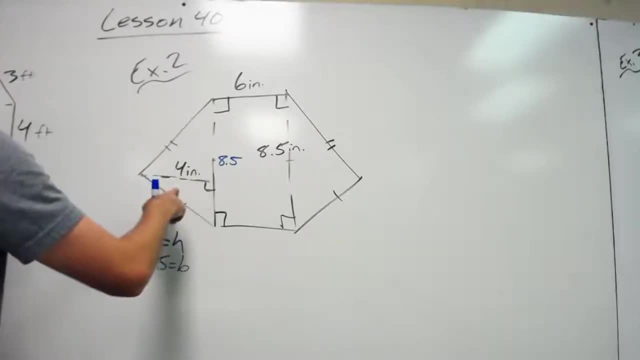 So now we can find the area of this triangle. Now notice: these two triangles are congruent because of side, side side. All right, 1,, 2, 3. Because these two sides are congruent and we already know that 8.5 is here. 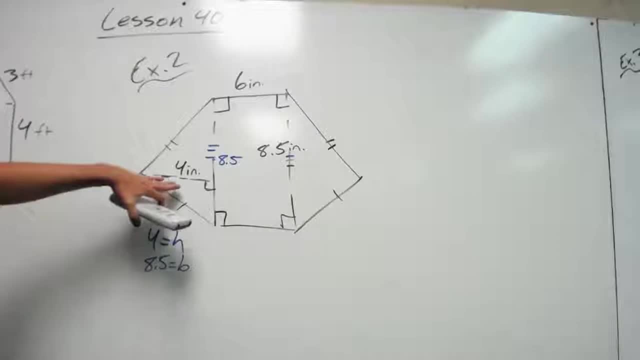 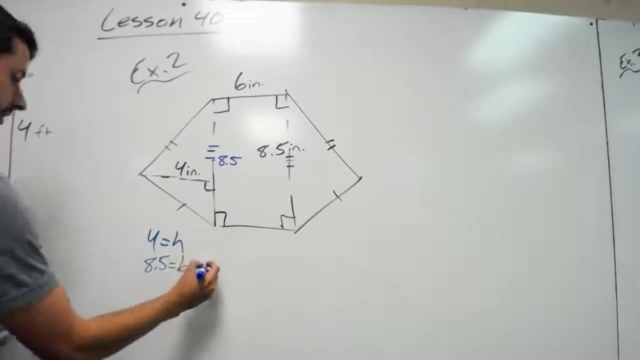 We know that side side side congruency. Once we find the area of this triangle, we can just multiply it by 2, because it's also the area of this triangle. They're the same, So I plug this into our formula. 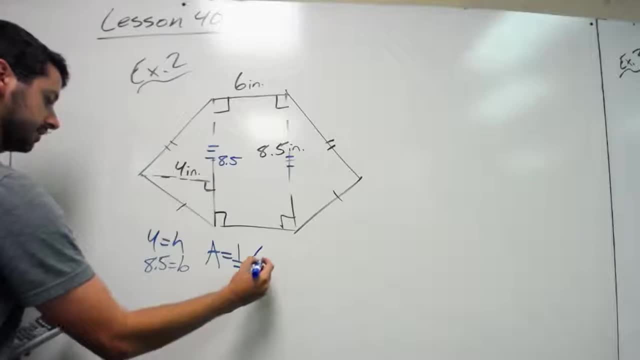 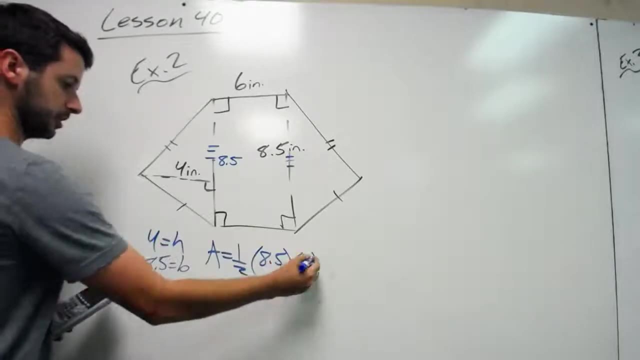 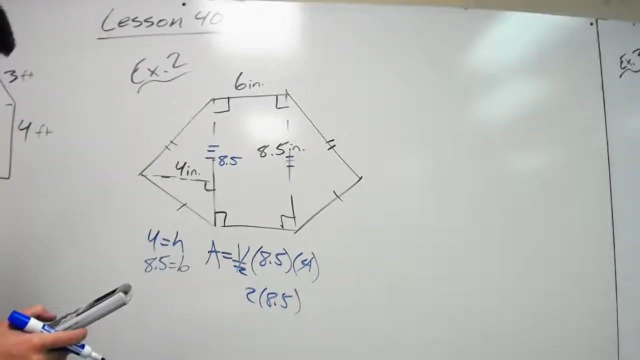 Area equals 1 half base, 8.5 times height, 4.. Area of a triangle: 1 half of 4, is 2.. So we're left with 2 times 8.5.. Multiply that and get 17.. So the area of this triangle is 17,, making the area of this triangle also 17.. 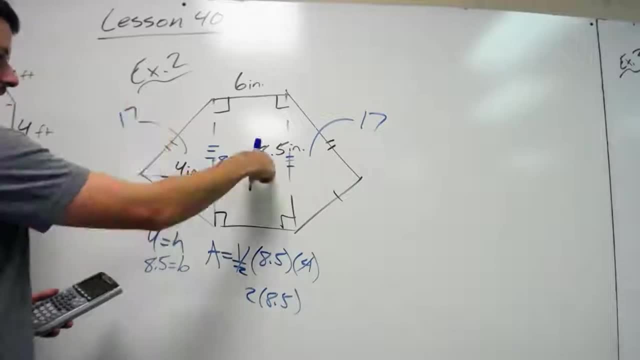 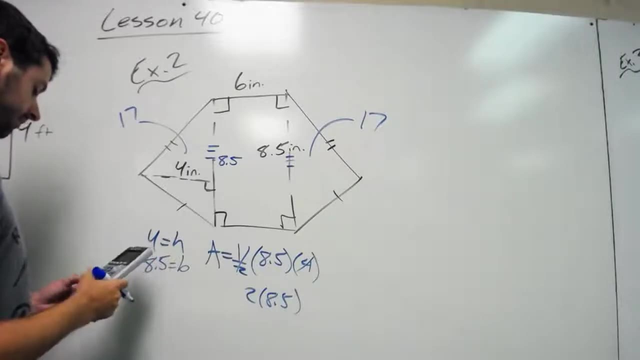 Now we just have to find the area of the rectangle. We have the height of 8.5, base of 6.. So we simply, for quadrilateral, we multiply base times height, 8.5 times 6. And we get 51.. 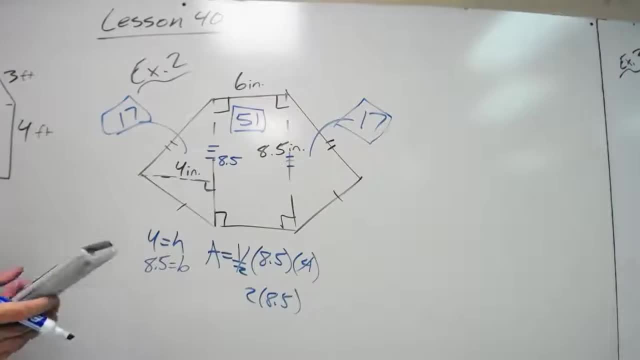 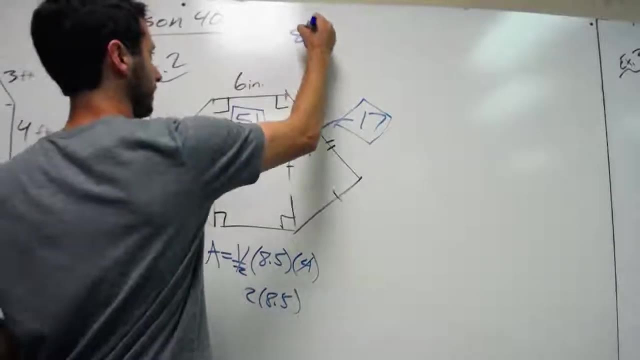 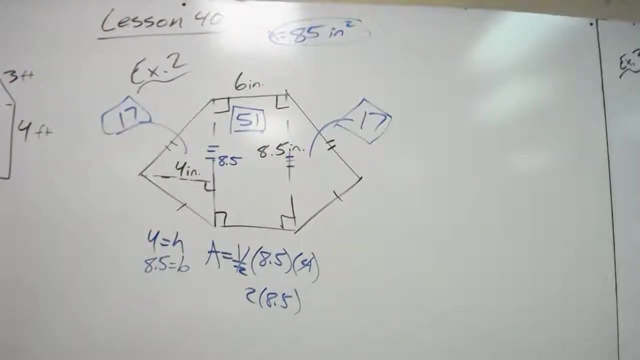 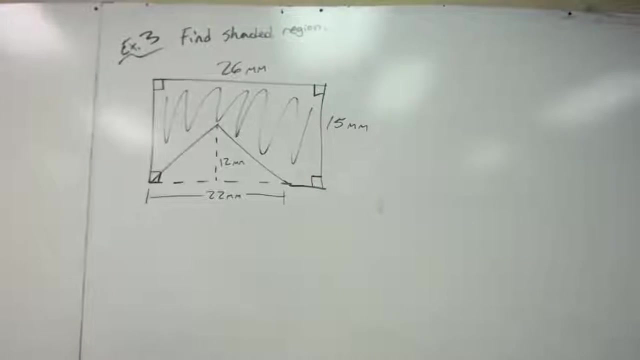 So now that we have all those, we add them together, We do 17 plus 51 plus 17 to get our area of 85 inches squared Equals our area. Now let's look at one different type of composite figure here. It wants us to find the area of the shaded region in this composite figure. 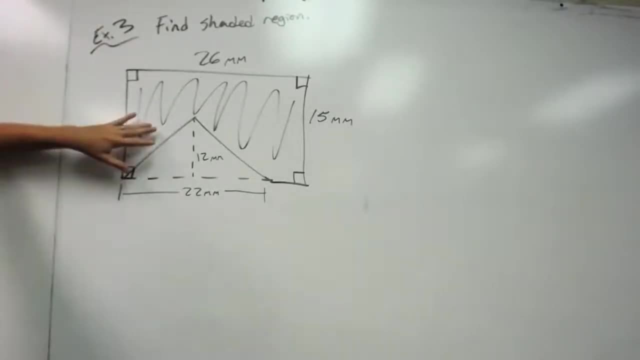 The last one, we would just find the area of the whole thing. Well, this one is a square with a triangle inside of it. So how do we find the area of this shaded region? Well, what we need to do is find the area of the total. 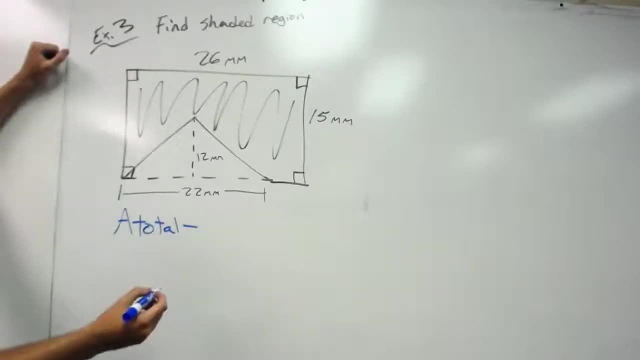 and then subtract the or. sorry, let me think about how I'm wording this. Yeah, the area of the total minus the area of- well, in this case the triangle. So I'm just going to put triangle. Really it's the figure inside. 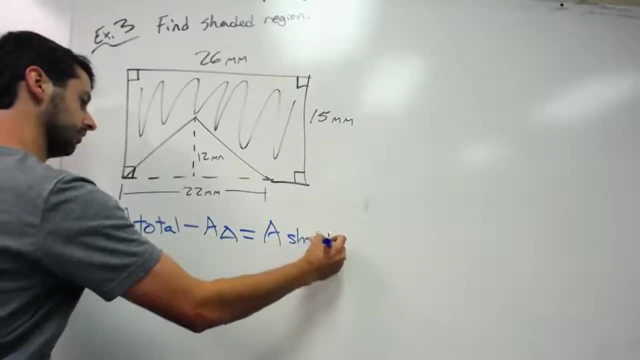 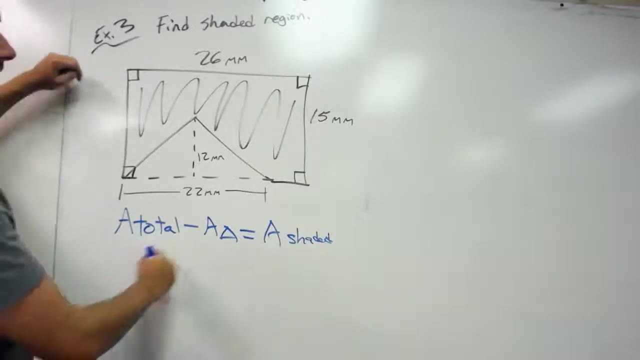 Equals the area of the shaded region. So let's first find the area of the total. Well, our total figure, or polygon, is a rectangle And it has a base of 26 and a height of 15.. So to find this, we're going to do 26 times 15.. 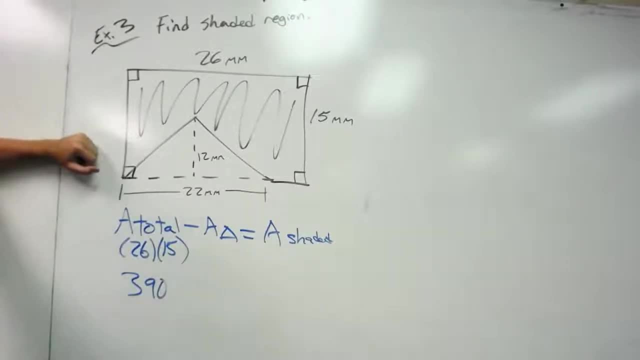 And we get 390 for the total area. Make that zero clear. Now we need to find the area of the triangle. Well, we have a height of 12.. That's perpendicular, That's our height. It just gives us the base of 22.. 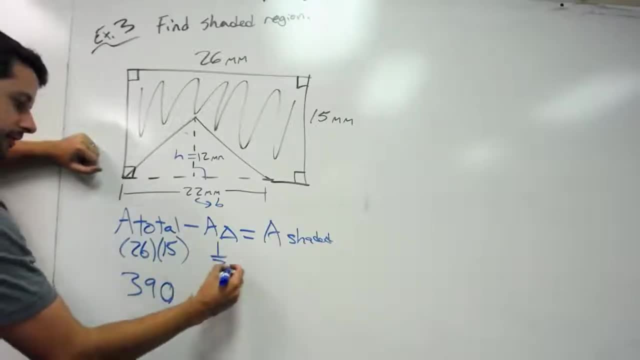 So we plug that into our formula of 1 half base 22 times height 12.. 1 half of 22 is 11.. So 11 times 12, however you want to put it in your calculator, That area is 132..